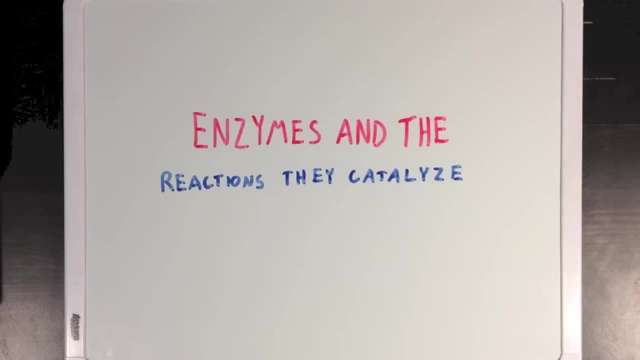 So today we're going to talk about enzymes and all the different kinds of reactions that enzymes can catalyze. But before we do that, let's review the idea that enzymes make biochemical reactions go faster, And if you look at a reaction coordinate diagram, you'd notice 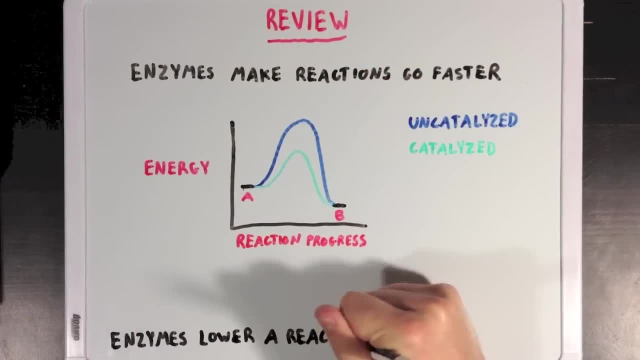 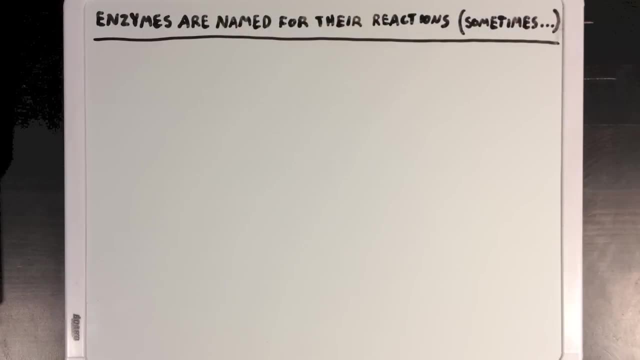 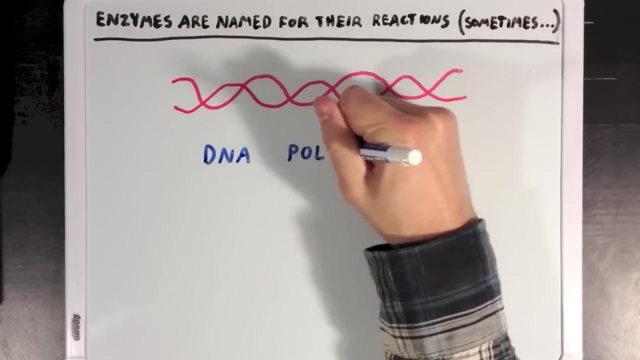 that enzymes speed up reactions by lowering their activation energy. Now, enzymes are generally named for their reactions, which is convenient, because it makes it a lot easier to remember what an enzyme does if someone gives you its name, And a great example of this is that one of the enzymes involved in DNA replication is called DNA polymerase. 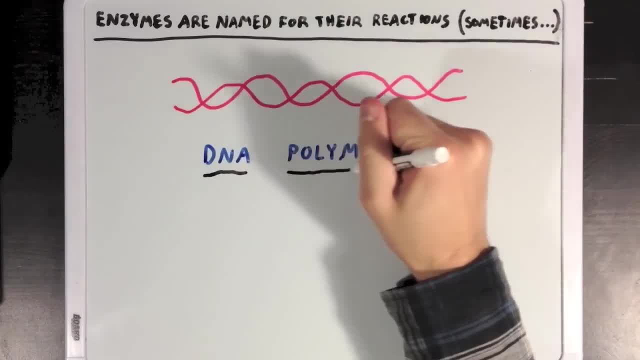 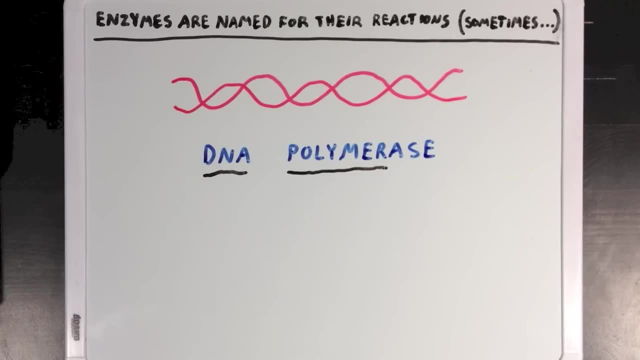 which is named as such because it acts on DNA and specifically makes polymers of DNA. Now, the suffix "-ase-" is usually just one that you find at the end of most enzyme names. Now, another great example is that, the enzyme that catalyzes the first step of glycolysis, 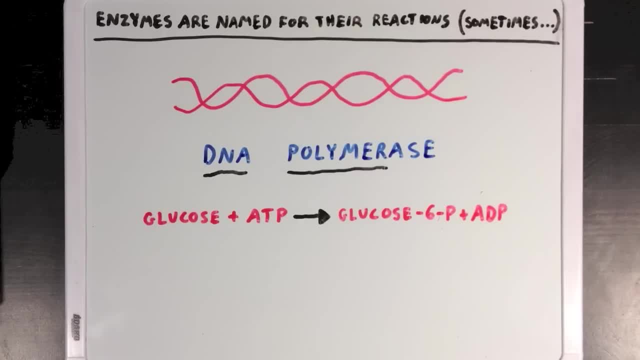 which you may remember, as the reaction between glucose and ATP to form glycogen is called hexokinase, And hexo refers to the number 6, which is a reference to glucose being a 6th carbon sugar, and kinase is a term referring to enzymes that add phosphate functional groups. 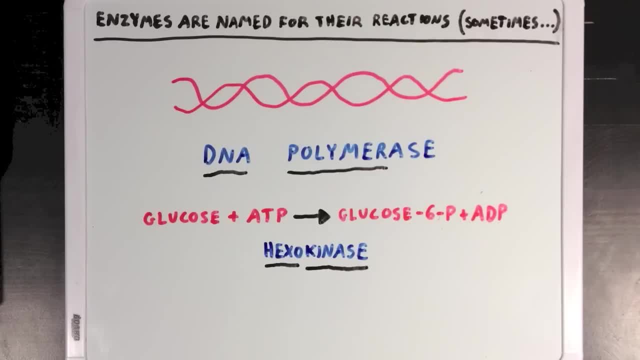 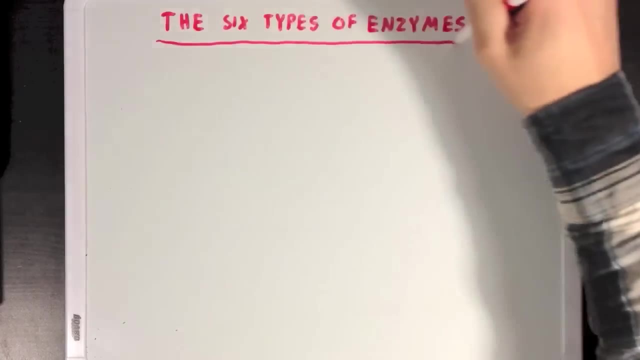 to different substrates. So overall hexokinase adds phosphates to 6th carbon sugars like glucose. Now, generally every enzyme has a very specific name that gives insight into the specific reaction that that enzyme can catalyze. So we can actually divide most enzymes into 6 different categories based off the kinds. 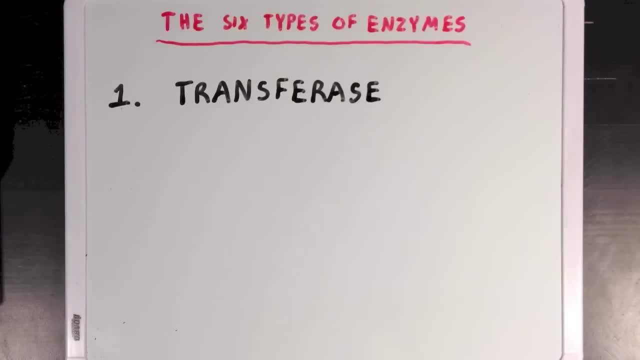 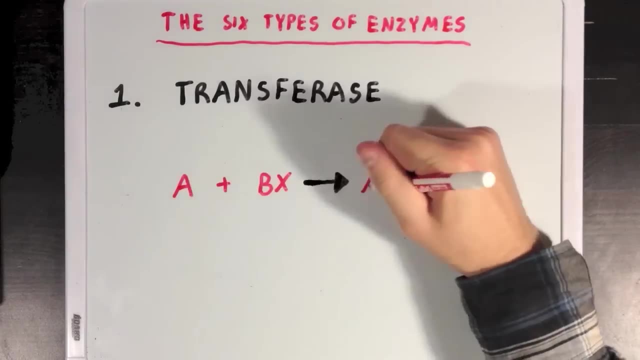 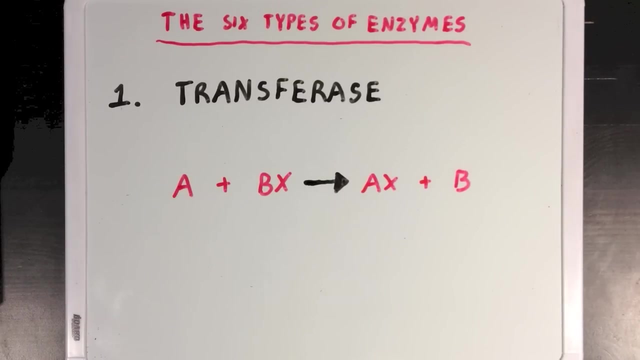 of reactions that they catalyze. Now our first group is the transferase group, And the basic reaction that transferases catalyze are ones where you move some functional group X from molecule B to molecule A, And a great example of one of these reactions occurs during protein translation, where amino acids bound. 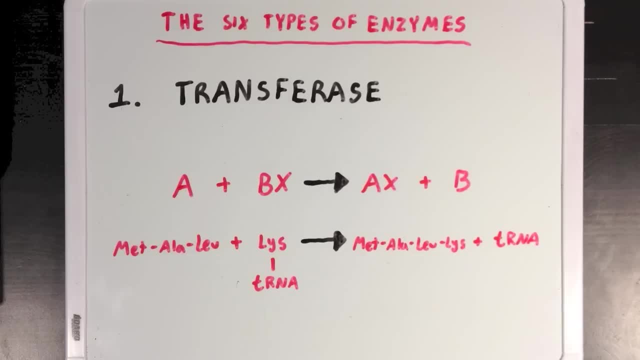 to tRNA molecules are transferred over to the growing polypeptide chain. So, in this case, A refers to our amino acid chain, B refers to our tRNA and X refers to this lysine residue which is being transferred from B to A And this reaction in particular. 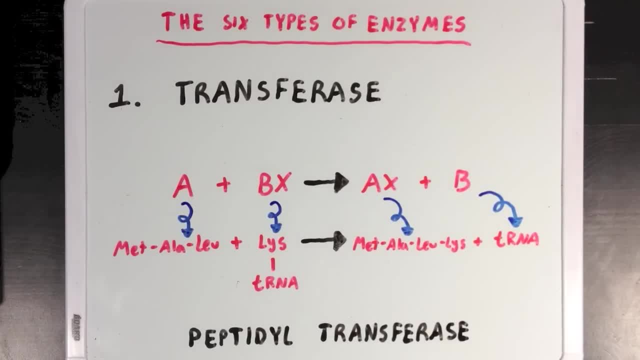 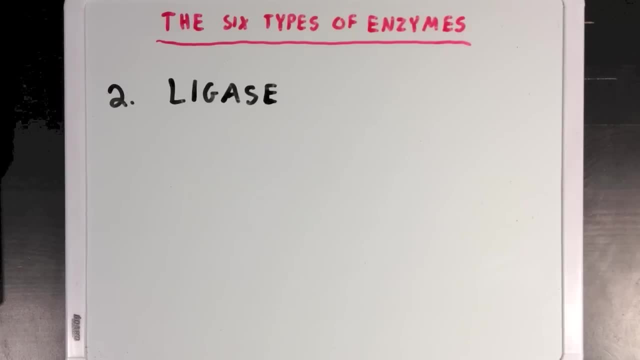 is catalyzed by an enzyme called peptidyl transferase, which is an appropriate name since it is a transferase involved in making peptides. Next we have the ligase group, which catalyzes reactions between two molecules, A and B. 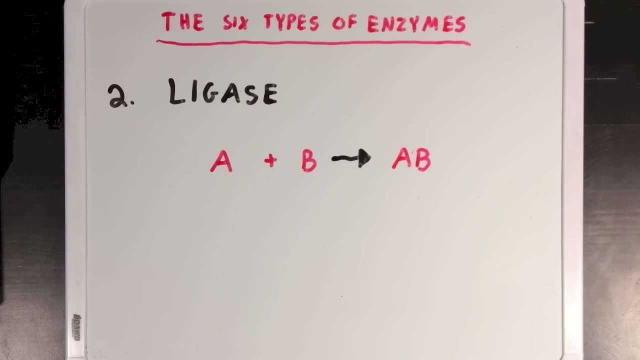 that are combining to form a complex between the two or AB, And an example of a reaction using a ligase that you might be familiar with occurs during DNA replication, where two strands of DNA are being joined together. So in this reaction, A and B represent the two separated DNA polymers which are being 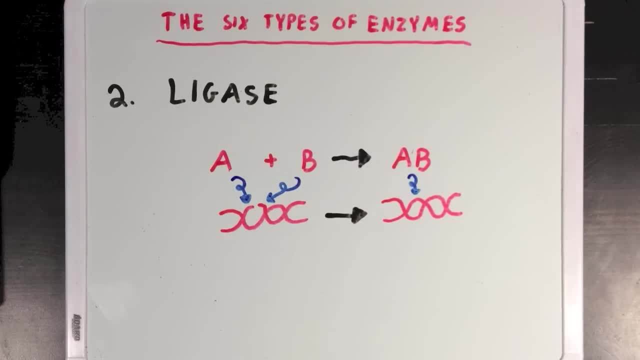 joined to form a single strand, And this reaction, in particular, is catalyzed by an enzyme called DNA ligase, which is named since it is a ligase that works on DNA strands. Now our third group is the oxidoreductase group. 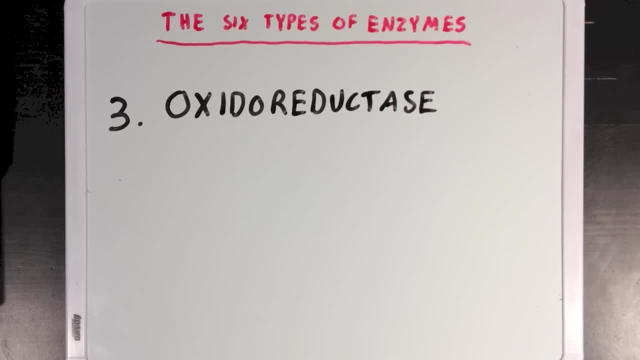 Which is a little different from the others, since it actually includes two different types of reactions, And these reactions involve transferring electrons from either molecule B to molecule A or from molecule A to molecule B. Now we say that an oxidase is directly involved in oxidizing. 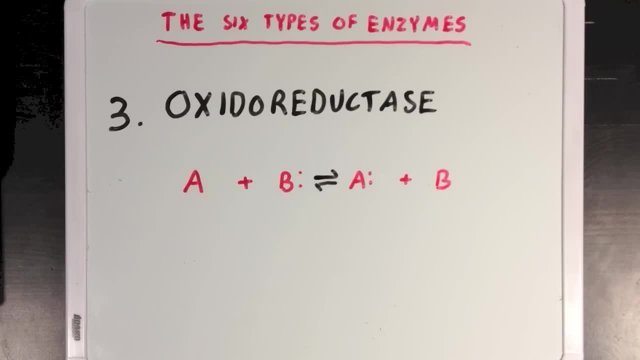 or taking electrons away from a molecule, while a reductase is involved in reducing or giving electrons to a molecule, And we call these enzymes oxidoreductases together, because they can usually catalyze both the forward and the forward, And this is why I've used equilibrium arrows here instead of just a normal single-headed. 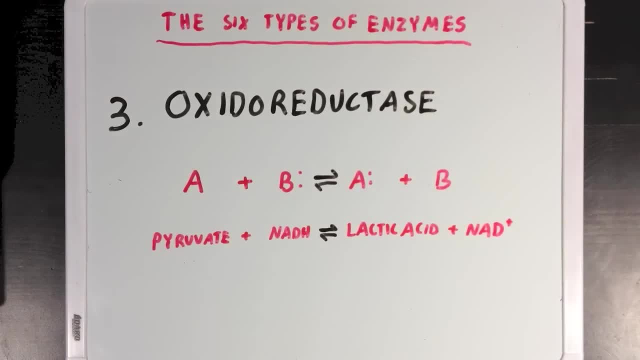 arrow. Now, a great example of an oxidation reduction reaction occurs during lactic acid fermentation, where electrons are either passed from NADH to pyruvate or from lactic acid to NAD. Now this reaction is catalyzed by an enzyme called lactate dehydrogenase. 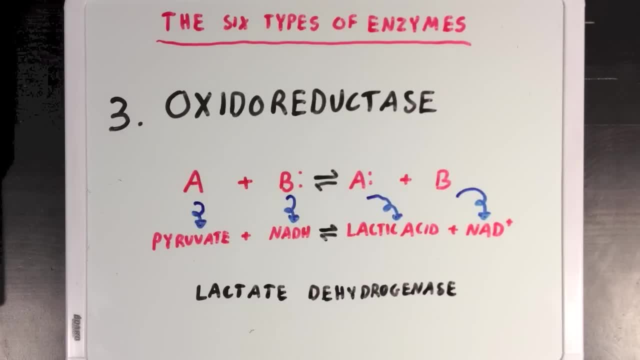 Remember that the word dehydrogenase refers to the removal of a hydride functional group, And that's the same as saying the removal of a hydride functional group. It's basically the removal of electrons, since hydrides are basically just hydrogen. 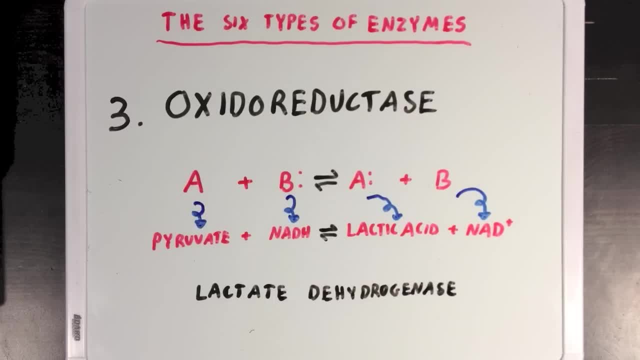 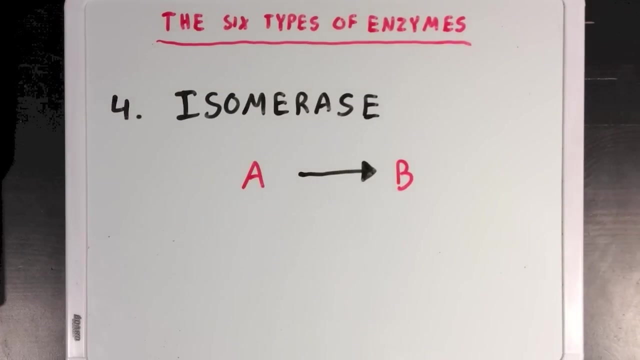 atoms with two electrons on them instead of just one. Now, this enzyme is given its name since it's able to remove a hydride or remove electrons from a molecule of lactic acid. Next we have the isomerase group, And enzymes in this group are typically involved in reactions where a molecule like molecule. 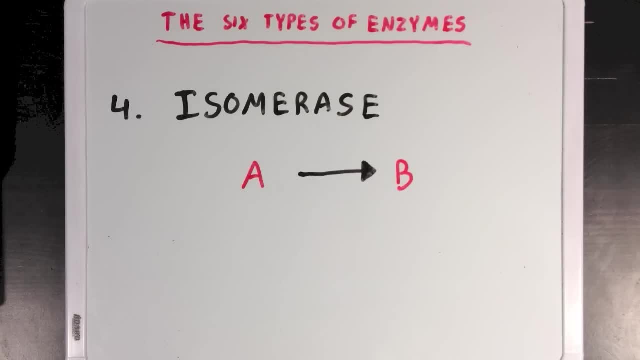 A is being converted to one of its isomers, And an example of this type of a reaction is the conversion of glucose 6-phosphate. Glucose 6-phosphate to fructose 6-phosphate, which is one of the steps of glycolysis that 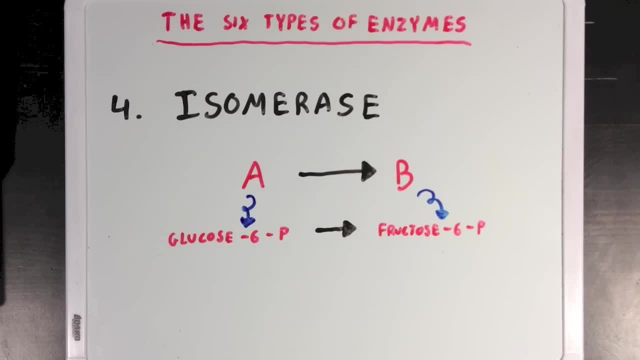 you may remember Now, this reaction is catalyzed by an enzyme called phosphoglucose isomerase, which is appropriately named, since it creates isomers of glucose molecules that are phosphorylated. Now our next category is the hydrolase category. 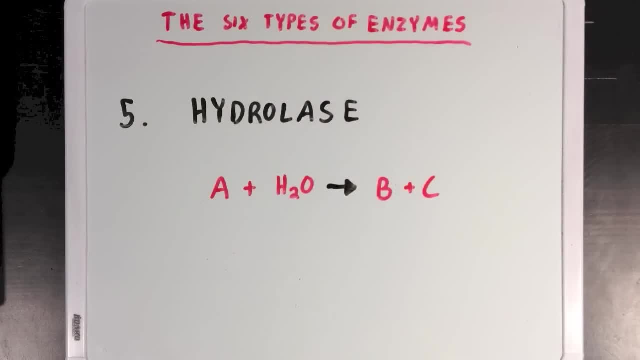 And hydrolases use water to cleave a molecule like molecule A into two other molecules, B and C, And a great example of one of these reactions is the hydrolysis reaction that can occur to peptide bonds, And if we have this lysine-alanine dipeptide here, it could be reacted with water to form. 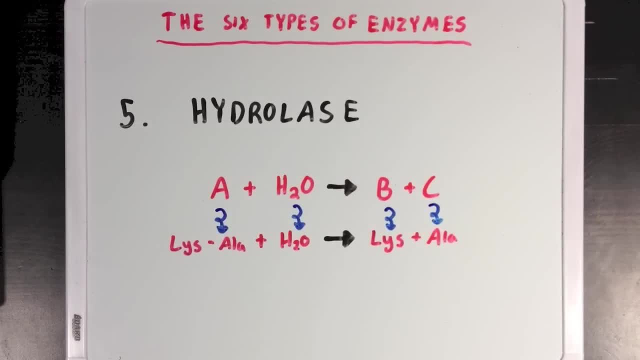 two individual amino acids that are no longer bound, And this particular hydrolysis reaction can be catalyzed by a class of enzymes that we call serine hydrolases, which some people call serine proteases, And they are named this way because they are hydrolases. 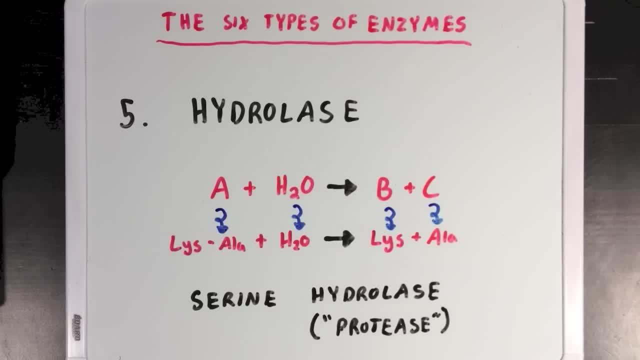 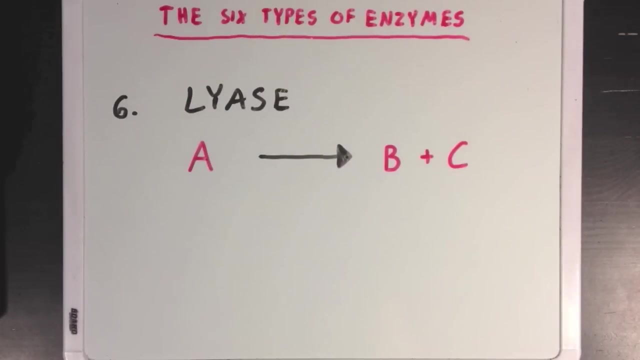 And serine residue is the key catalytic amino acid that is responsible for breaking the peptide bond. Now, our last category is a little more complicated than the others, And it's the lyase group. Now, lyases catalyze the dissociation of a molecule like molecule A into molecule B, and 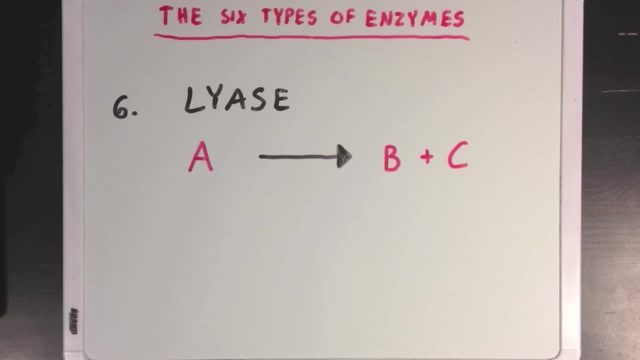 C without using water, like hydrolases would, and without using oxidation or reduction, like an oxidoreductase would. And one example of a reaction catalyzed by a lyase is the cleaving of a molecule A into an argininosuccinate, into arginine and succinate. 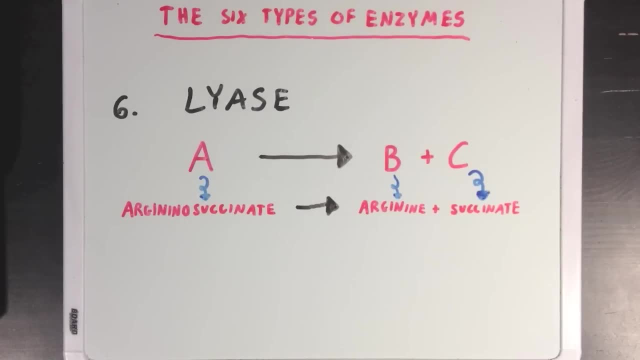 And this reaction takes place during the urea cycle, which you also might be familiar with. Now, this specific reaction is catalyzed by an enzyme called argininosuccinate lyase, which is appropriately named because it is a lyase that catalyzes the breakdown of an 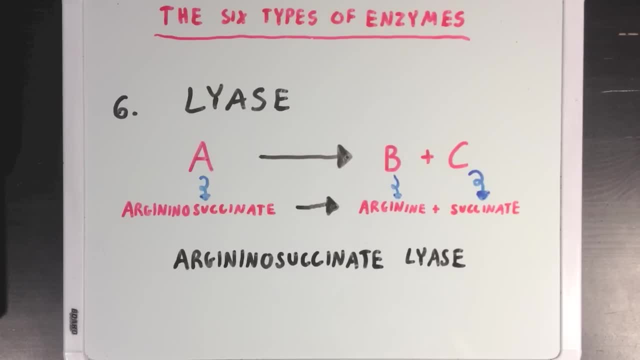 argininosuccinate molecule. Now it's important to recognize that, since lyases don't use water or oxidation to break a bond, they need to generate either a double bond between the two, or a double bond between two atoms or a ring structure in a molecule in order to work. 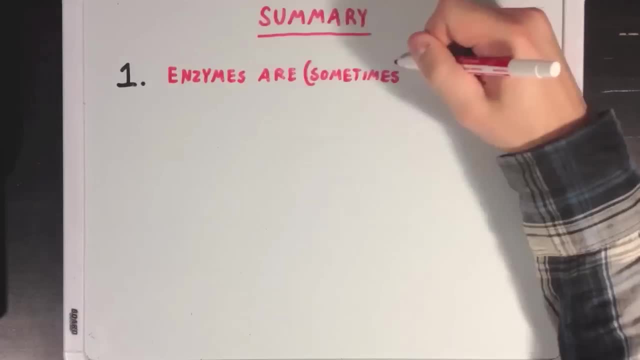 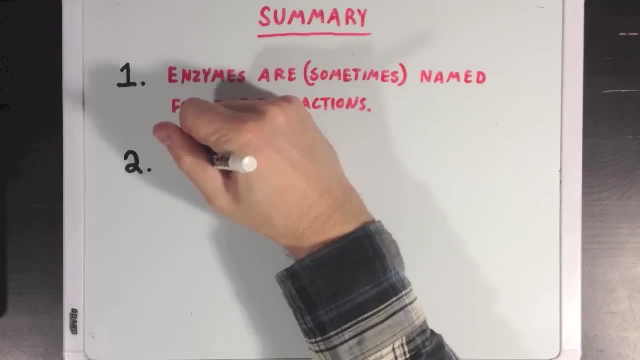 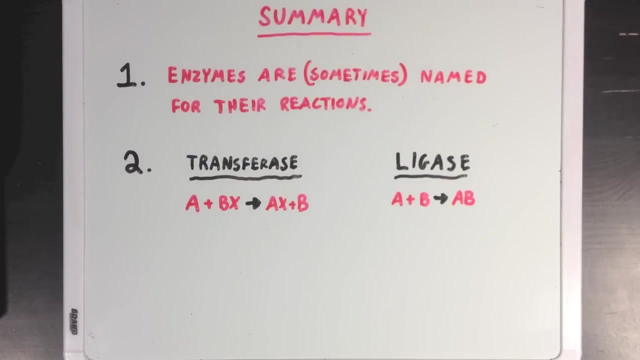 So what did we learn? Well, first we learned that enzymes are sometimes named for their reactions, And next we learned about the six different types of enzymes We have: transferases, which transfer functional groups from one molecule to another. ligases, which ligate or join two molecules together. oxidoreductases, which move electrons between. 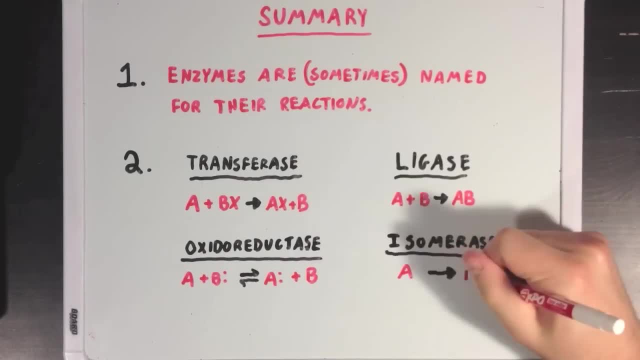 molecules: isomerases, which convert a molecule from one isomer to another, and oxido-reductases, which convert a molecule to another. hydrolases, which break bonds using water, and lyases, which break bonds without using water and without using oxidation. 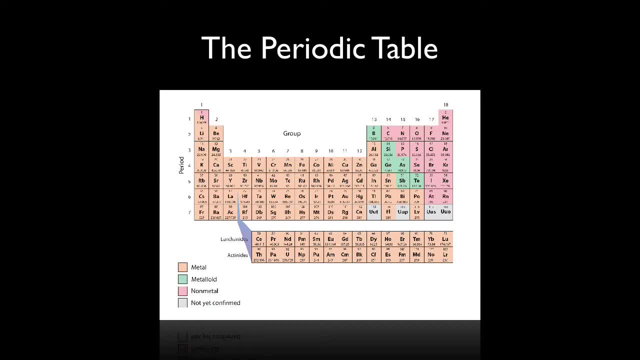 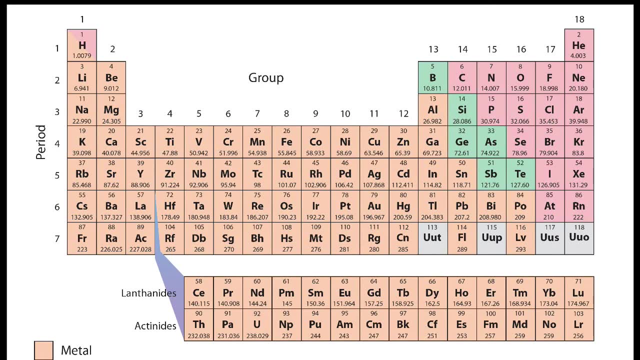 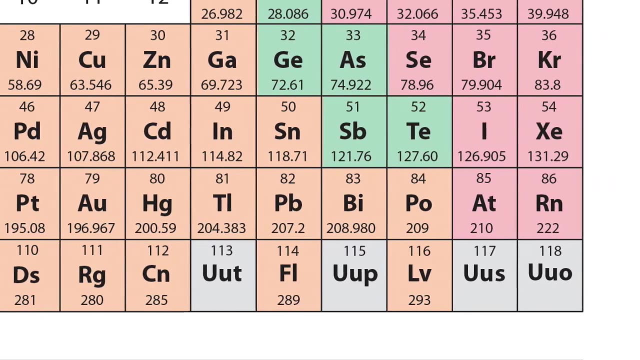 The periodic table is a listing of all the known elements. How many known elements are there? Just over a hundred. You'll hear in the news periodically of the discovery of a new element That's likely one of these heavier elements located around here in the 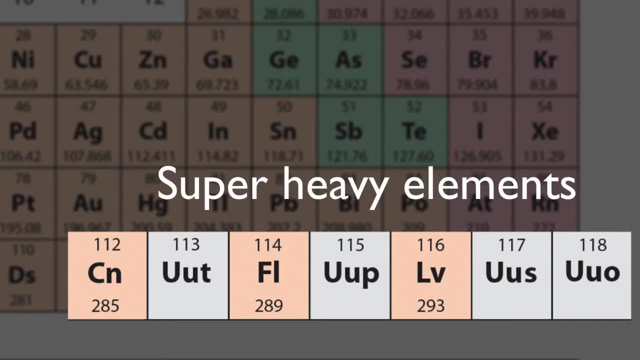 periodic table. As it turns out, these super heavy elements are so highly unstable that they exist for only a fraction of a second. These are all synthesized in the laboratory. You won't find any of these occurring in nature. The heaviest element that occurs in 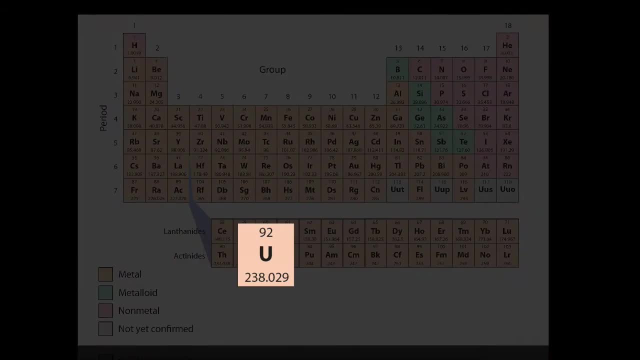 nature in any appreciable amounts. is uranium right here, number 92.. That's right. the periodic table lists the elements by their atomic number, which, you'll recall, is the count of the number of protons in the nucleus of each atom. Hydrogen has one proton, so 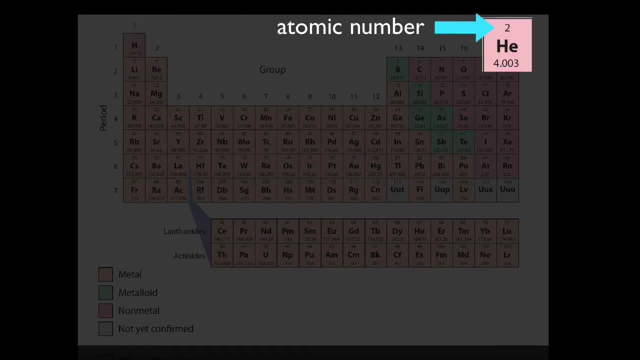 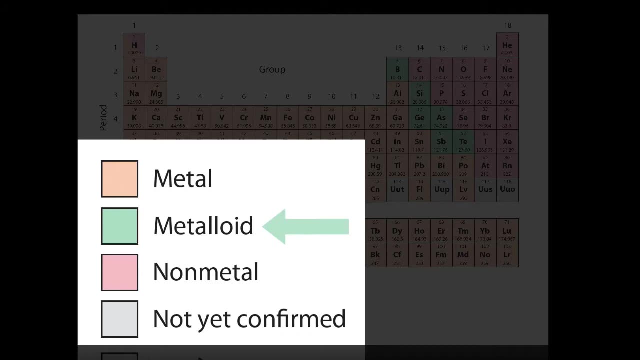 it's number one. Helium has two protons, so it's number two, and so forth. There are three types of elements: metals, nonmetals and the metalloids, which have both metallic and nonmetallic properties. As you can see, most elements of the periodic 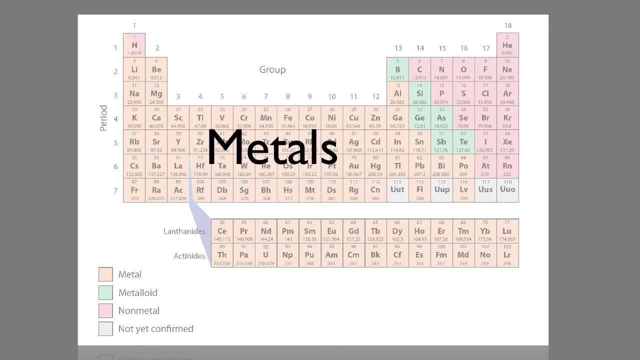 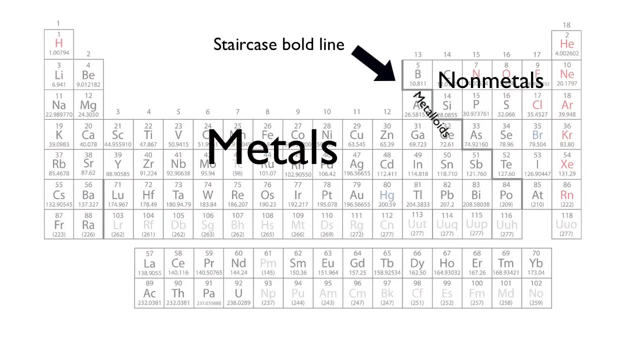 table are metals. They're grouped here naturally toward the left side. The fewer nonmetals are grouped to the upper right and, as is fitting, the metalloids fall right in between the metals and nonmetals. On the periodic tables you'll see the staircase bolt line that divides the metals. 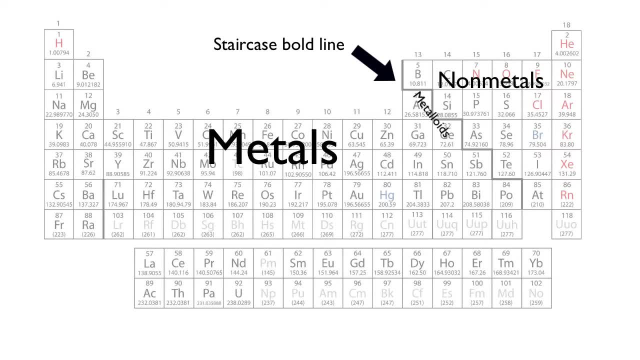 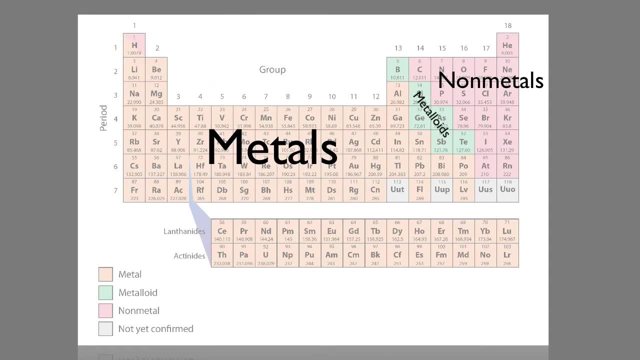 from the nonmetals. All the metalloids hover adjacent to this staircase bolt line, But because there's a gradual shift from metals to nonmetals, I prefer this view. Metals are great at conducting electricity. With few exceptions. nonmetals are just the.